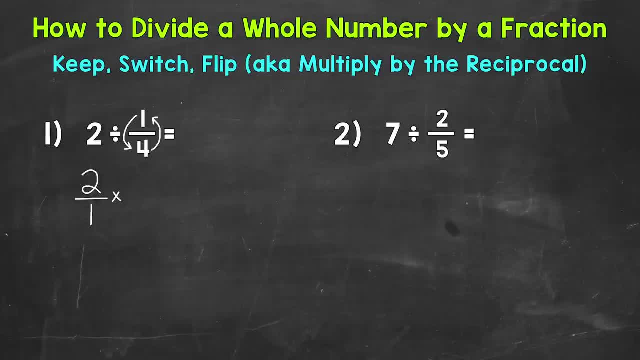 now going to be the numerator, and the numerator is now going to be the denominator, So we have four over one. Once we get to this point, we have a multiplying fractions problem, which we just multiply by one. So we have four over one. So we have four over one. So we have four over one. 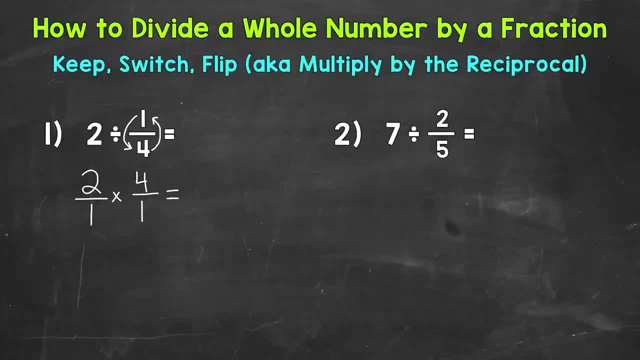 So we get to the answer of eight over one, which is an improper fraction, So we do not want to leave it like that. This is going to be eight. Our final answer is eight. Two divided by one fourth equals eight. Let's move on to number two, where we have seven divided by two. 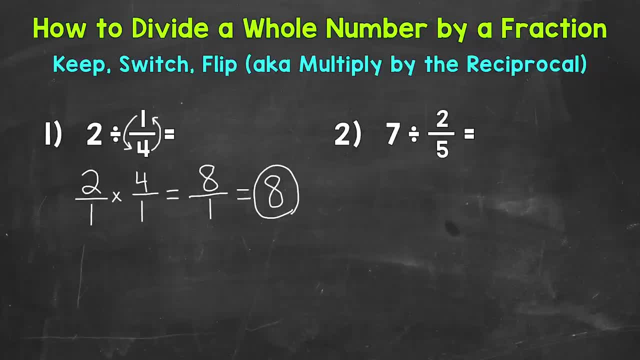 So we are finding out how many two fifths are in seven, so to speak. So keep, switch, flip. We will keep our seven, but put it in fractional form by putting it over one, switch to multiplication and then flip our second number or fraction. Now we can multiply straight across Seven times five. 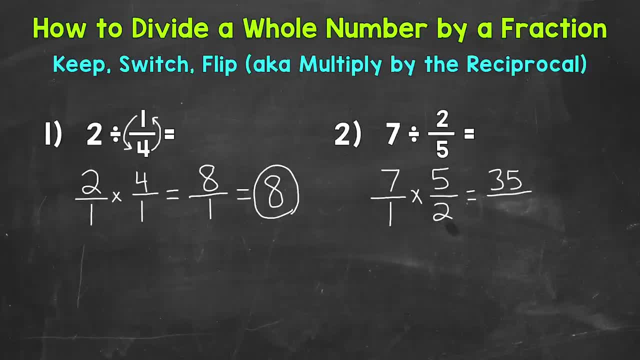 is thirty-five, And one times two equals two, So our answer is thirty-five over two. Now we don't want to leave it improper. We want to convert this to a mixed number. So we do: thirty-five divided by two. How many whole groups of two are in thirty-five? Well, seventeen, So that's our whole number of our mixed 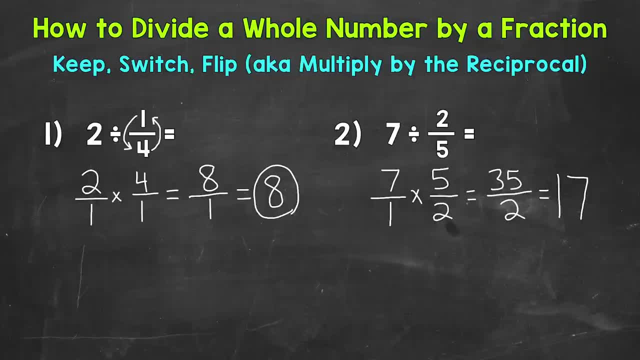 number Now. we didn't hit thirty-five exactly, We had a remainder of one, So we have one over two. We have a remainder of one, So that's our numerator of the fractional part, And then we keep our denominator of two the same, So seventeen and a half Always. look to see if you can simplify the. 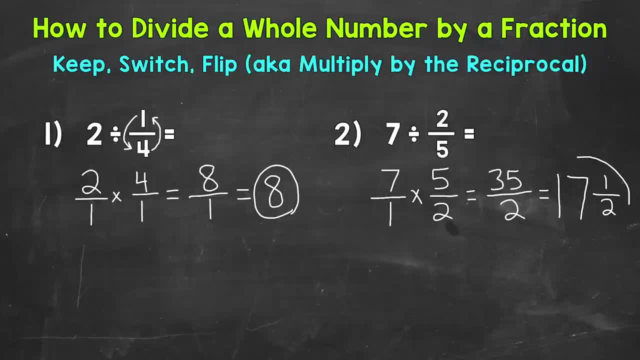 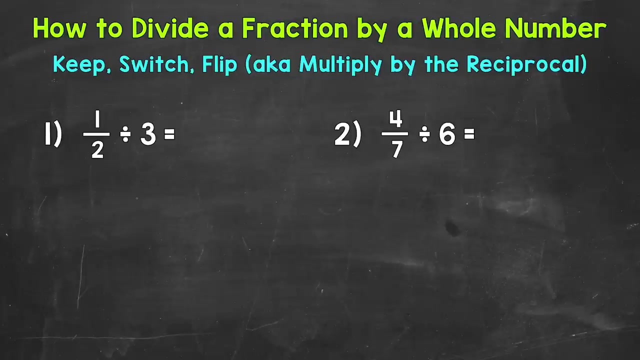 fractional part One half is in simplest form. So we are done. Our final answer: seventeen and a half. So that's how we divide a whole number by a fraction. Let's move on to dividing fractions by whole numbers. So here are our examples for dividing fractions by whole numbers. Let's jump into number one, where 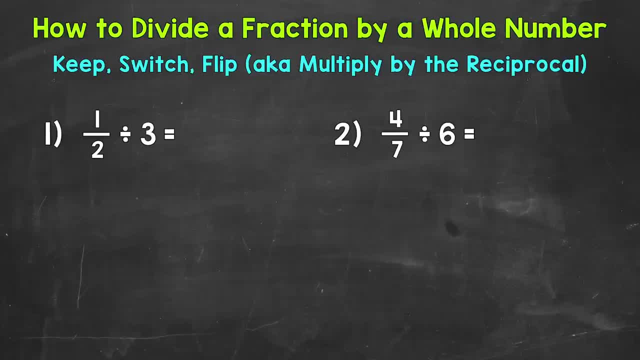 we have one half divided by three. So we are taking one half and dividing it into three equal groups or parts. Let's rewrite the problem using keep switch flip in order to solve this. So always keep the first fraction or number. So let's rewrite the problem. So one half, we are going. 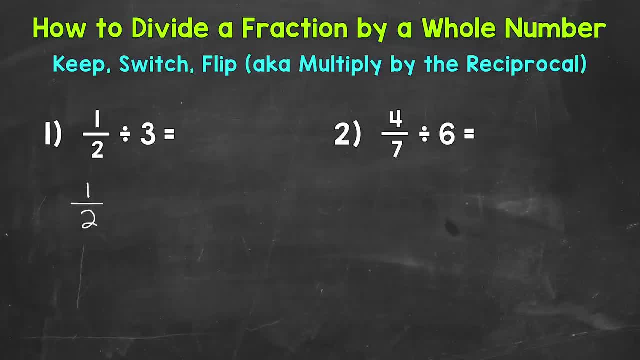 to keep. Then we switch to the opposite or inverse of division, which is multiplication. And since we switched to multiplication, we need to flip the second number or fraction. In the case of number one, we have a whole three here. So how do we flip this? Well, let's put that whole number over one. 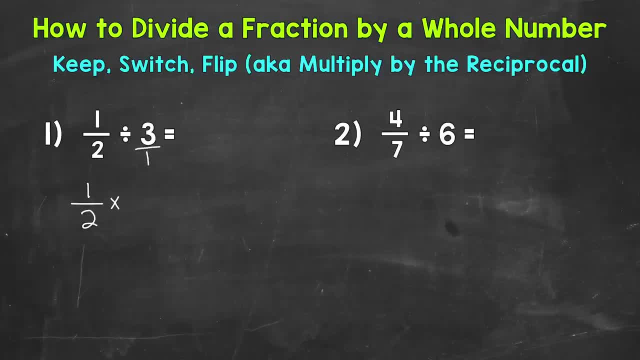 That way we have a numerator and a denominator That does not change the value of the whole number. The problem that still has a value of three. So now we can flip, So the one is going to go up to the top and be our numerator And the three is going to be the denominator. So we flipped that. second, 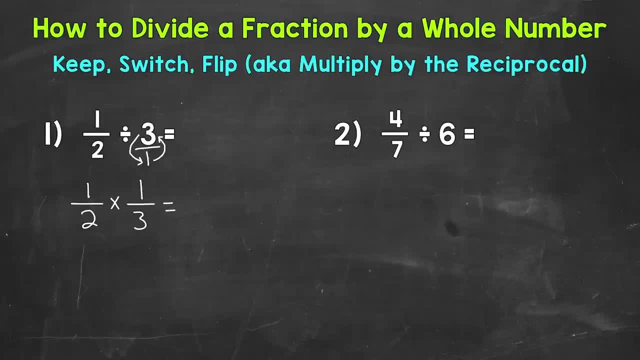 number. Once we get to this point, we have a multiplying fractions problem. So we can multiply straight across: One times one is one And two times three is six. So one sixth is our final answer. Always check to see if you can simplify. One sixth is in simplest. 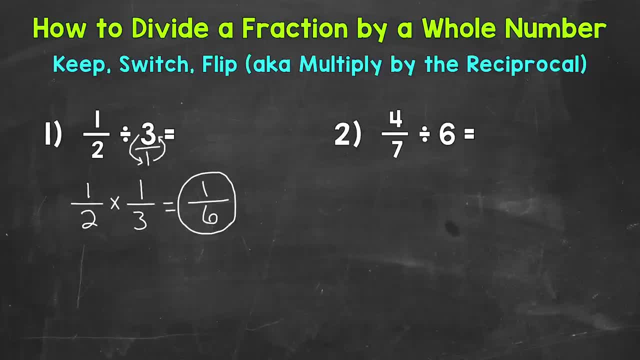 form. So we are done: One half divided by three equals one sixth. Let's move on to number two, where we have four sevenths divided by six. Keep, switch, flip. So let's rewrite the problem: Keep four sevenths, Switch to multiplication. 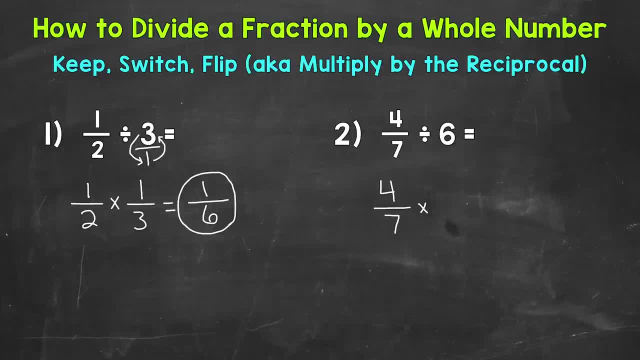 And then we need to flip, So we can write that six in fractional form. And now we can flip, So the one is now our numerator And the six is now our denominator, And we can multiply straight across: Four times one is four. Seven times six is forty-two, So we 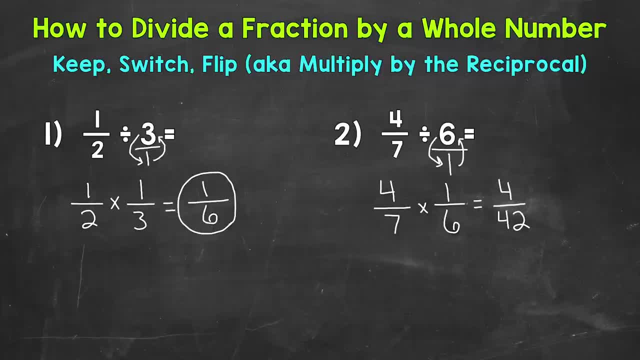 get four over forty-two, Which can be simplified. Four and forty-two have a greatest common factor of two. So let's divide each of these by two And we get two over twenty-one for our final simplified answer. And that's how we divide a fraction by a whole number. Lastly, we have fractions divided by fractions. 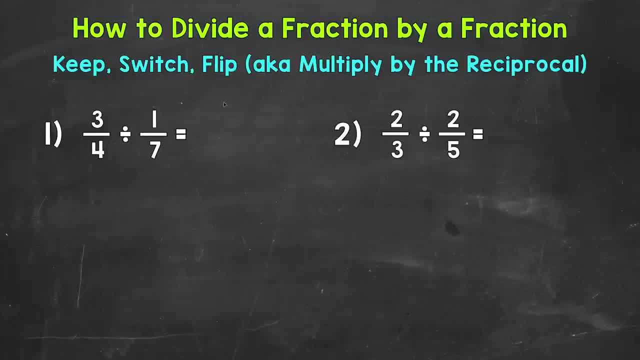 So let's move on to that. Here are our two examples for dividing fractions by fractions. Let's jump into number one, where we have three fourths divided by one seventh. So we are seeing how many one sevenths we can make out of three fourths, or how many one sevenths are in three. 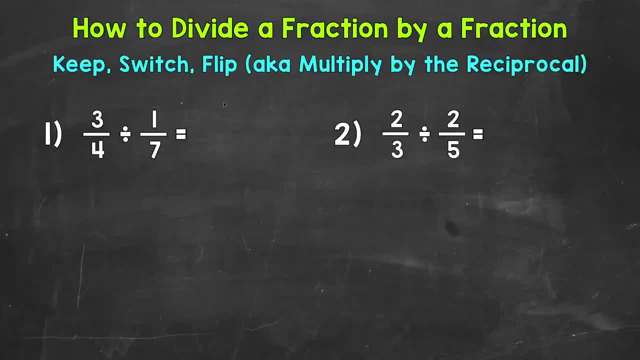 fourths, so to speak. So let's start by rewriting this problem using keep, switch, flip. So we always keep the first fraction or number, So we keep three fourths, as is We switch to the opposite or inverse of division, which is multiplication. And since we switch to the opposite or inverse, 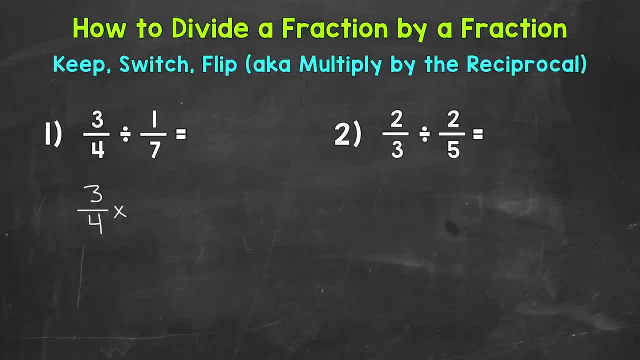 of division. we're going to flip the second fraction, So the seven is going to be our numerator and the one is going to be our denominator, So we end up with seven over one. Once we get to this point, it's a multiplying fractions problem. 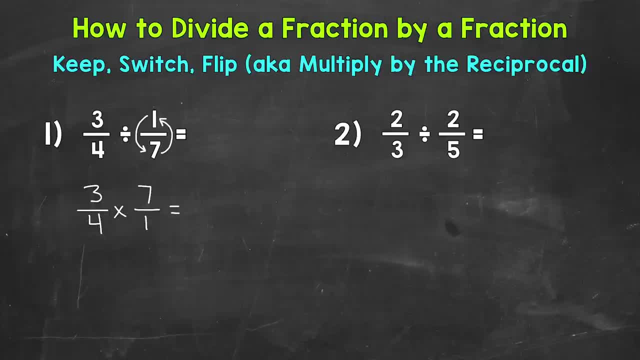 So we can multiply straight across: Three times seven is 21.. And then four times one is four, And we end up with 21 fourths. Now, that's an improper fraction, So we do not want to leave it. We need to divide our numerator of 21 by four. How many? 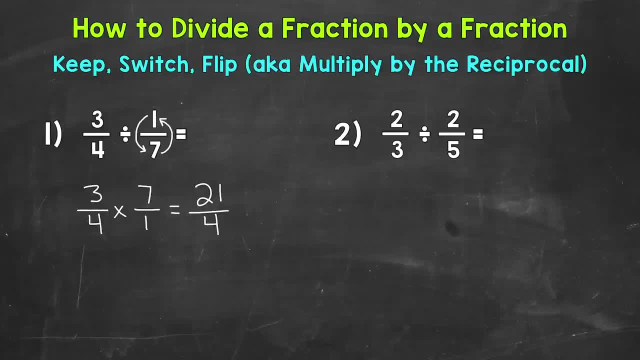 whole groups of four are in 21?? Well, five, That gets us to 20.. So five whole groups of four, That's our whole number of the mixed number here. Now that doesn't hit 21 exactly. We have a remainder.